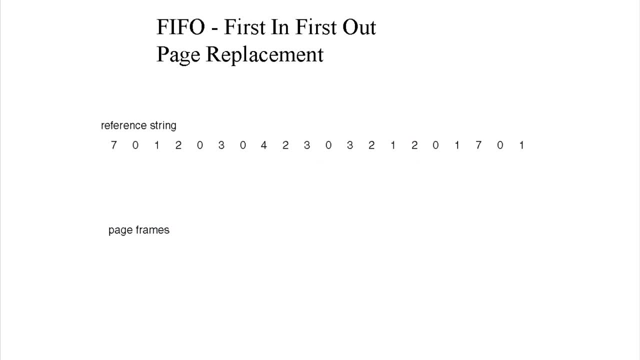 which is almost self-explanatory from the name itself. first in, first out. However, I find that it's easy to get lost in it and try to apply a most recently used, which is a completely different, algorithm for handling this scenario. But I will go ahead and 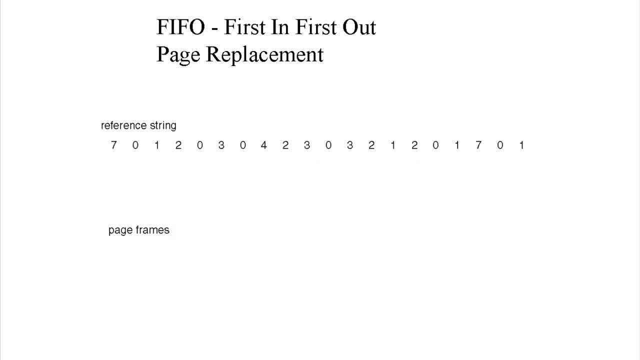 demonstrate in this example exactly how the first in, first out page replacement system, or algorithm rather, handles the page replacements. Okay, so let's get started. You'll see that the first page fall is actually going to be the 7, and then the 0 and the 1.. 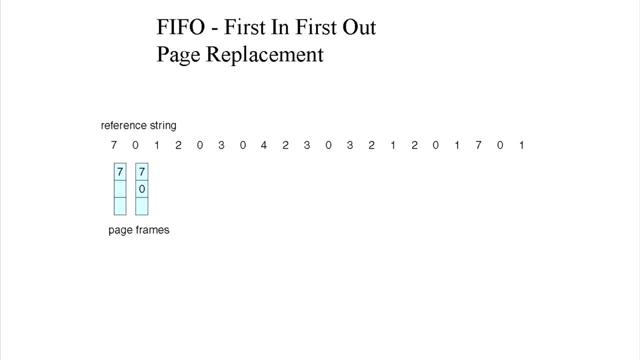 And the reason they're page falls is because they weren't already there. Basically, anytime you add a new value into the memory, it's considered a page fall because it wasn't pre-existing. So let's just add the 2.. And what's important here is this is the actual first replacement. 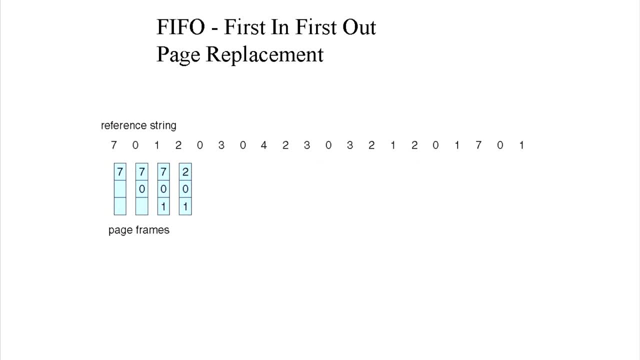 And if we just look at the page frames that we have currently, and rather than focusing on the reference string itself, if you just look at whichever number has been in there the longest, which is obviously the 7,, it's the one that was in first, So it's the one. 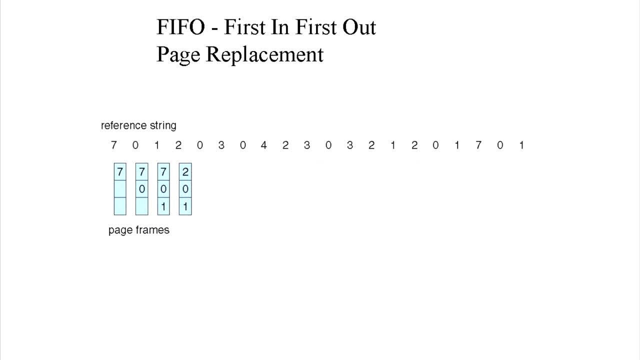 that needs to be replaced here As we continue on. the next number in the reference string is the 0. And because we already have a 0 inside of our memory here, we're going to not do anything there And we're going to move on to the number afterwards, which is: 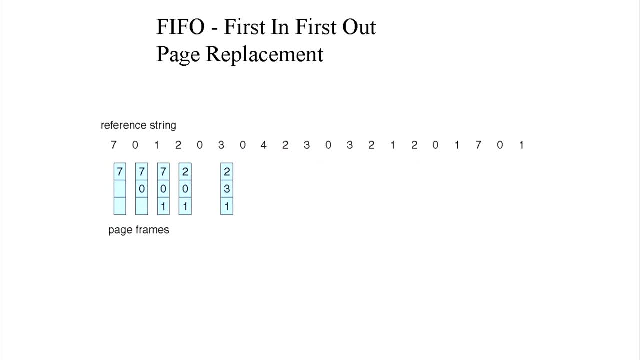 the 3. And it will, in fact, be replacing the 0, even though it seems like maybe the 1 should be replaced because the 0 just came up. That would be incorrect and it would be confusing it with the most recently used algorithm that I mentioned. 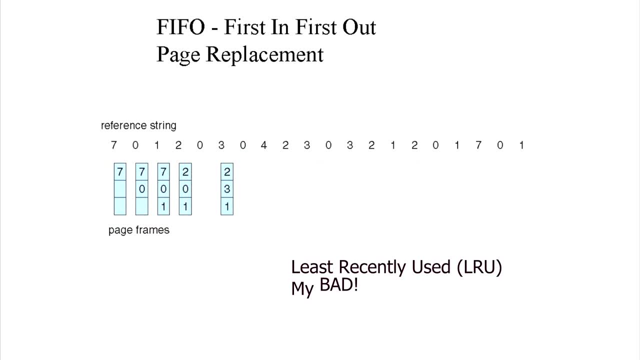 Now we have another 0, and if we look at our page frames, as I mentioned before, if we look at the number that's been in there the longest, which is the 1 now, since the 2 has only been in there for 3 frames and the 3 has only been in there for 1 frame, the 1